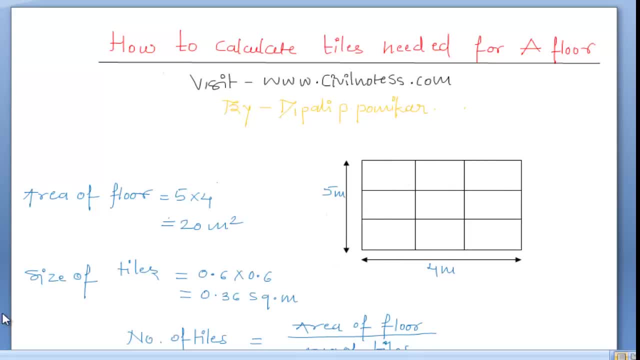 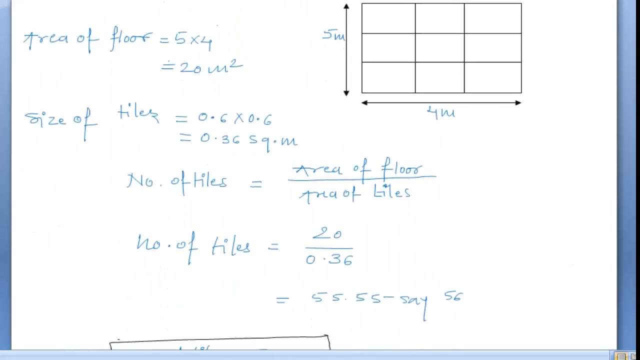 If we wanted to calculate the number of floors. so we know these. We know the standard size of tiles. The standard size of tiles is 0.6 into 0.6 meter square. So after that we have to calculate the area of tiles. We know the size of tiles. Just multiply with these two terms, that is, 0.6 into 2 number, 0.6 into 0.6.. We get the 0.36 square meter. This is the area of tiles. If we wanted to calculate the number of tiles, we know the formula of number of tiles. 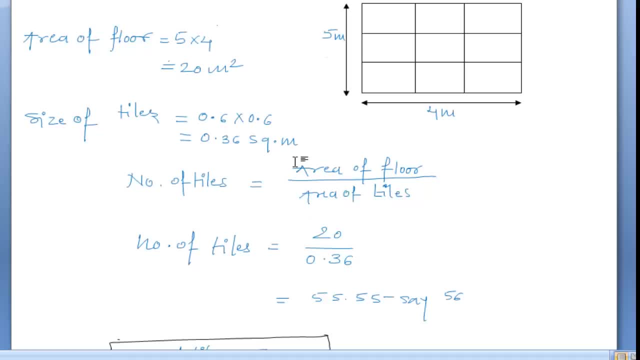 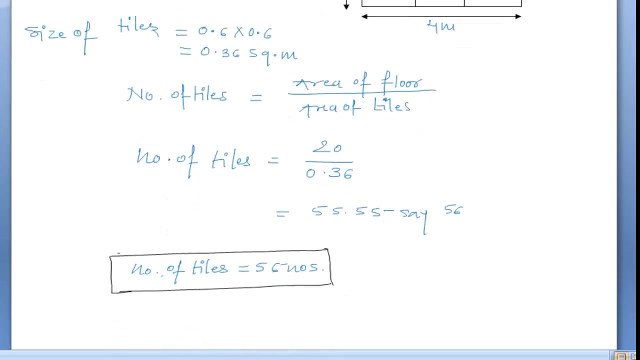 That is a area of floor upon area of tiles. We just calculated the area of floor and area of tile. Just put the answer and put the value and get the answer. That is, area of floor is 20 meter square and area of tiles is 0.36.. We get the number of tiles is 55.55 after this calculation, 20 upon 0.36.. Say it as a 56.. We get the number of tiles is 56.. In this area, this 5 into 4.. 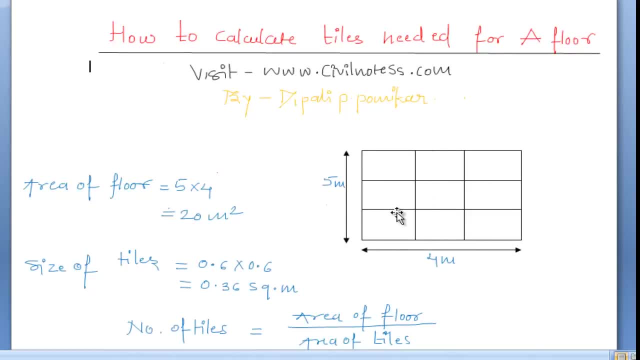 square area of floor. we know 56 number of tiles is fit in this area. okay, now you have to keep in mind some two notes. that is, if we are placing the tiles in a floor, then kept in a cure. cure means in a water before applying for of one. 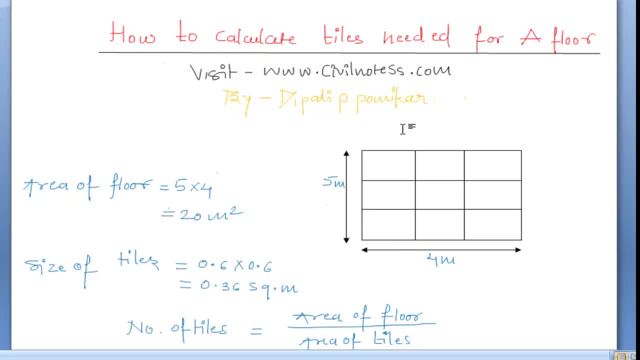 day, so that when we are placing it on the floor then it will never absorb the water from the cement pest. it will create a good bonding, okay then. second one is the if we are placing a tiles in our walls. first one for the if we are placing in the tiles in a floor, then second one is if we are placing the 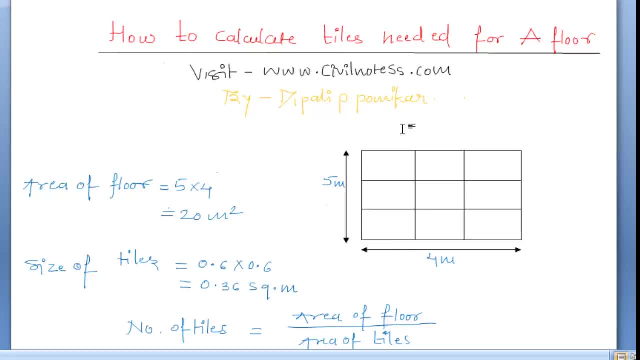 tiles in a wall, then make sure make, make a slurry of cement and apply it on the wall. that like a paint. so just we have to apply it on the wall after that like the paint and then place the tiles on wall so that it will create a good bonding with the wall and it will not create any any bad look okay.